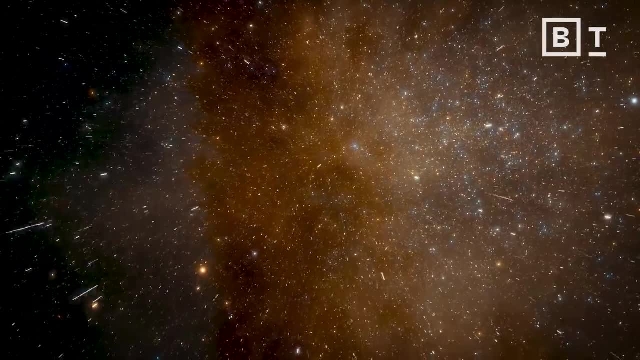 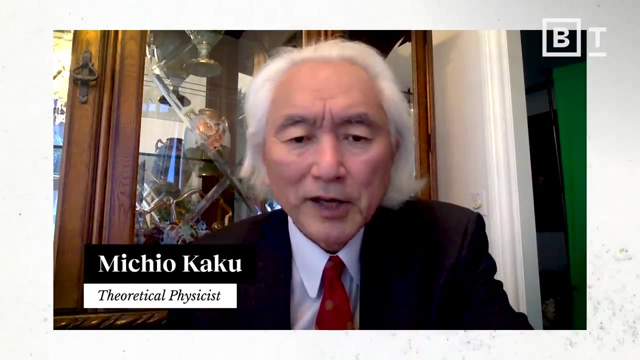 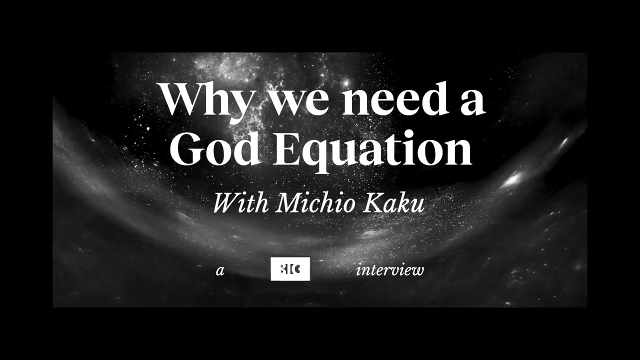 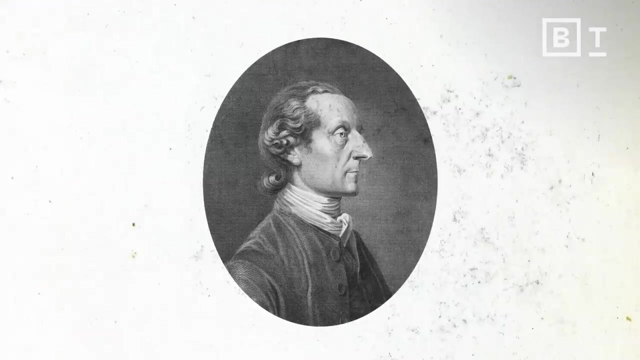 the God equation. My name is Professor Michio Kaku. I'm a professor of Theoretical Physics at the State University of New York and author of the recent book The God Equation: The Quest for the Theory of Everything. Leonard Euler, one of the great mathematicians of human history. 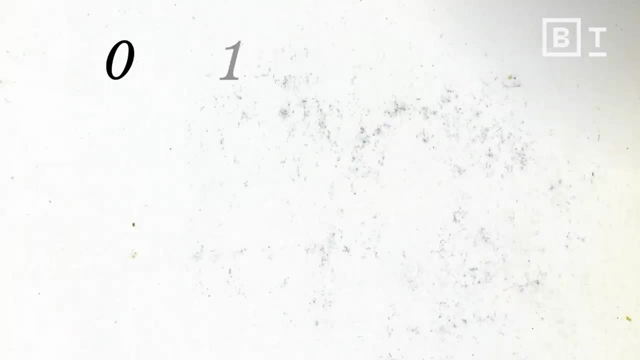 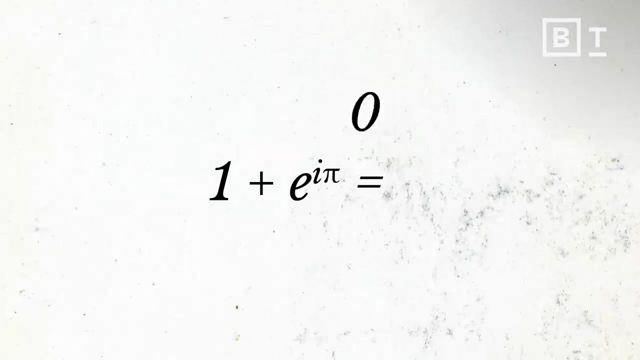 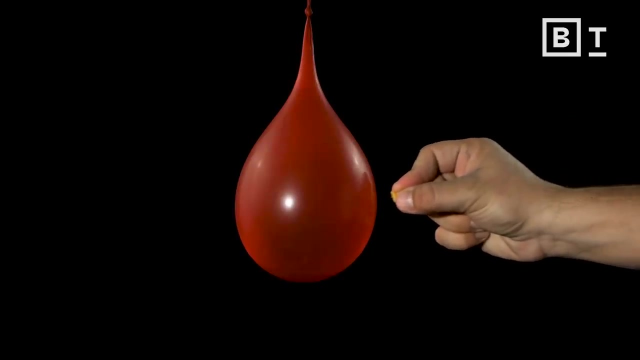 found one of the most important theories of everything, One equation which summarized the fundamental constants of math: One plus e to the i pi equals zero. People call that the God equation of mathematics. Now, of course, the God equation is useless as a practical application. 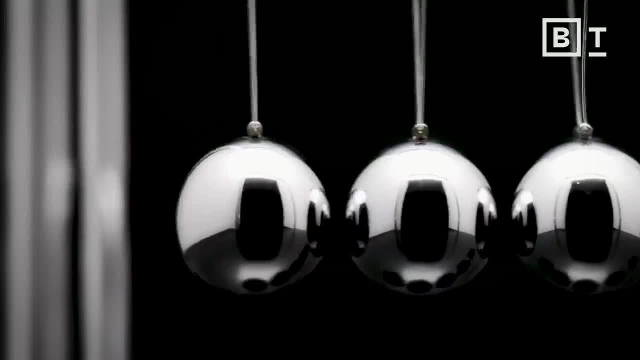 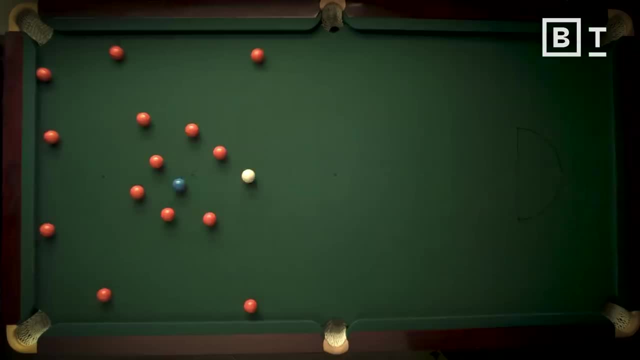 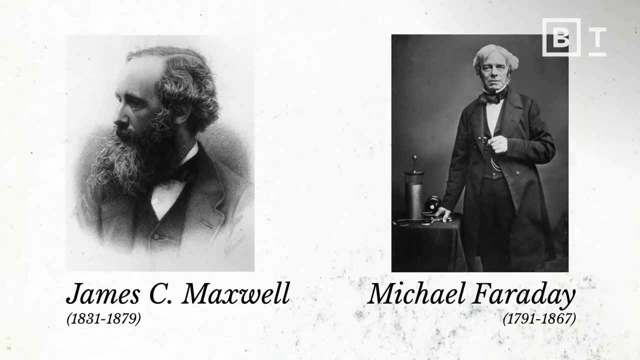 But think now of a God equation for physics. Physics is quite useful. When Newton worked out the mechanics of moving objects and gravity, he helped to lay the groundwork for the industrial revolution. And then Maxwell and Faraday united electricity and magnetism to give us 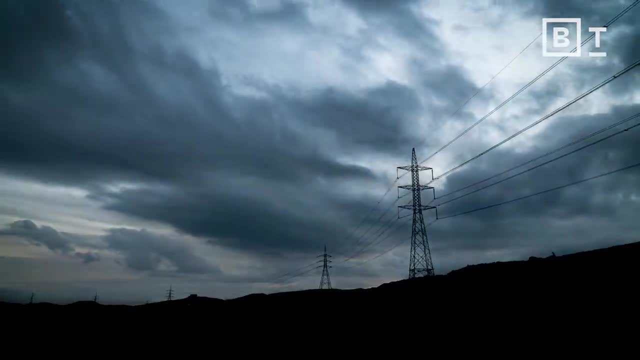 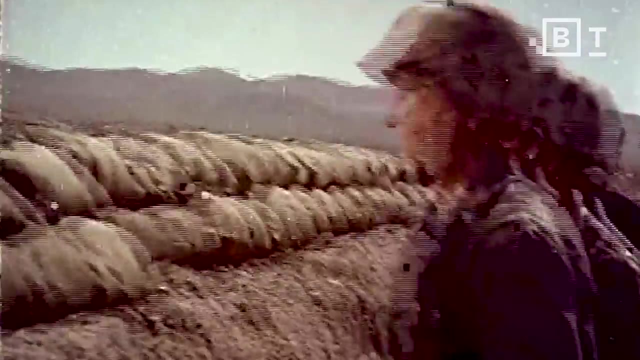 the electromagnetic force, the electric revolution of dynamos, generators and light bulbs. And now we have E equals mc squared, which helped to pave the way for the nuclear force. Each time a force was unraveled, it changed the course of the universe. 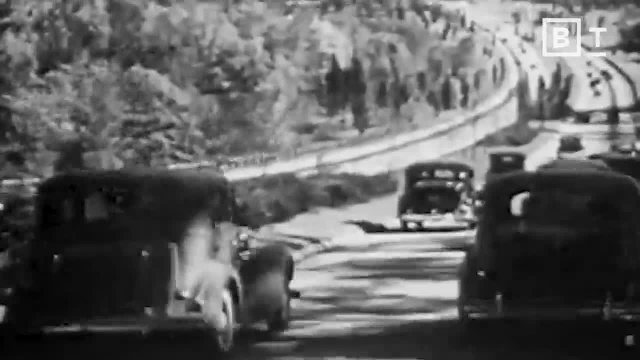 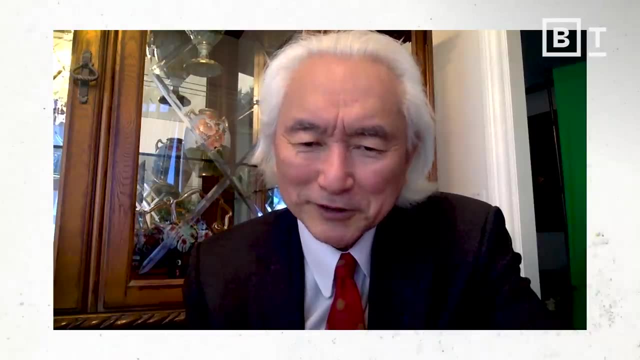 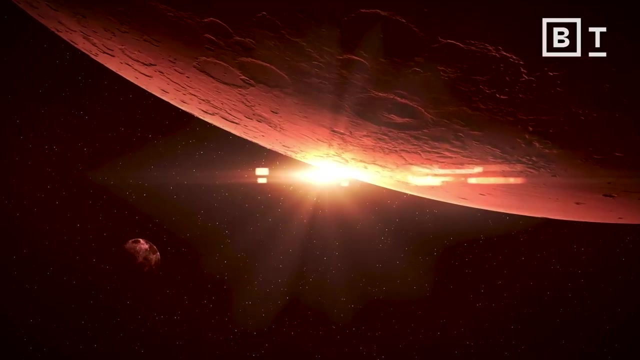 Each time a force was unraveled, it changed the course of the universe, human history. And now we want to put the whole thing together into the God equation, fulfilling Einstein's original dream. The God equation, just like the God equation of mathematics, should unify the basic concepts. 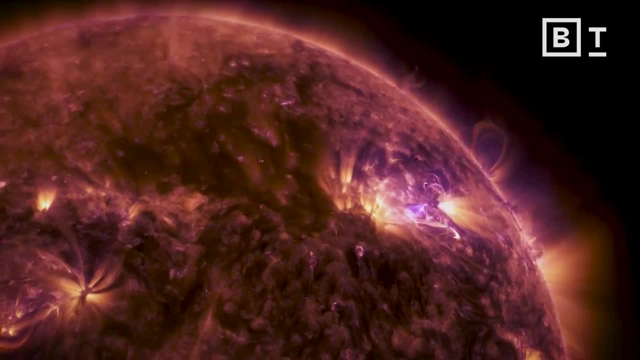 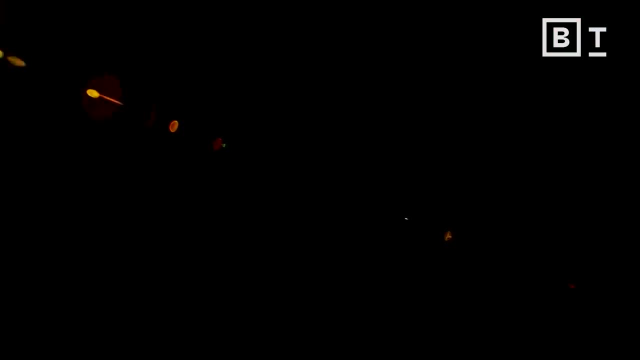 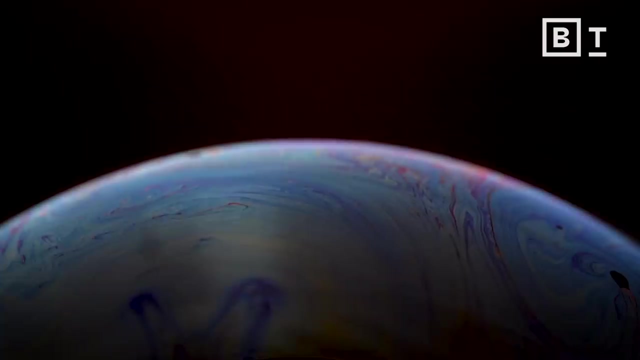 of physics into one equation. And what are these basic concepts? Relativity and the quantum theory. The problem is, the quantum theory does not unify well with general relativity. See general relativity of Einstein is based on smooth surfaces. The quantum theory, 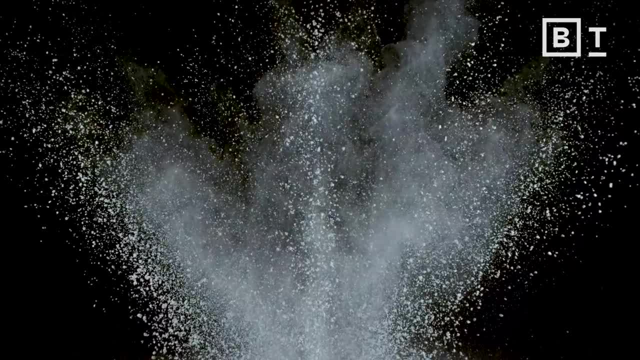 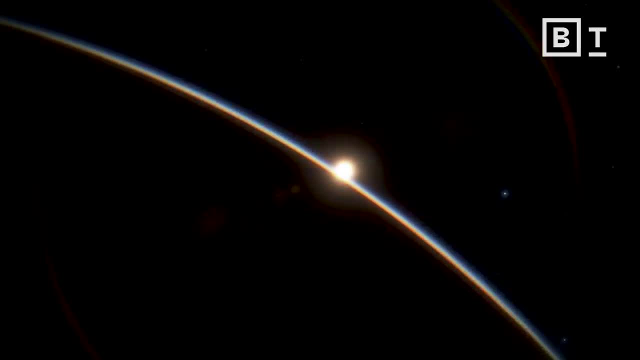 is based on chopping things up into particles. That's the opposite of Einstein's philosophy of smooth curves representing space-time. That's why it's so difficult. It's no exaggeration to say that the greatest mind in the world is the greatest mind in the world. It's the greatest mind. 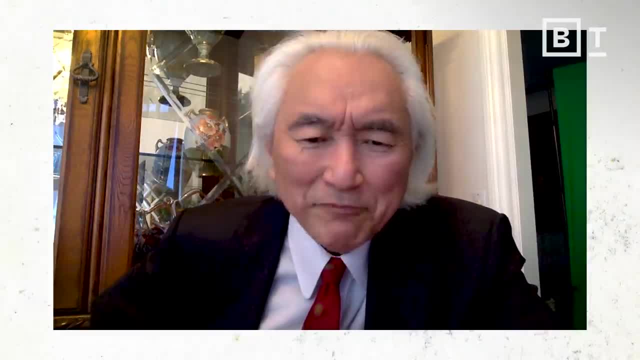 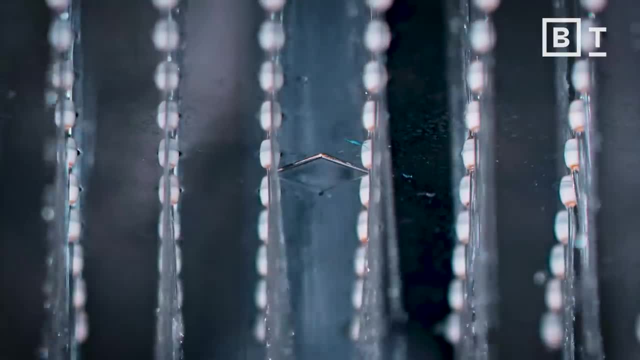 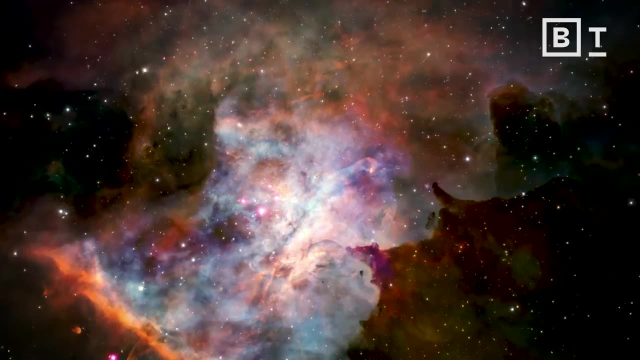 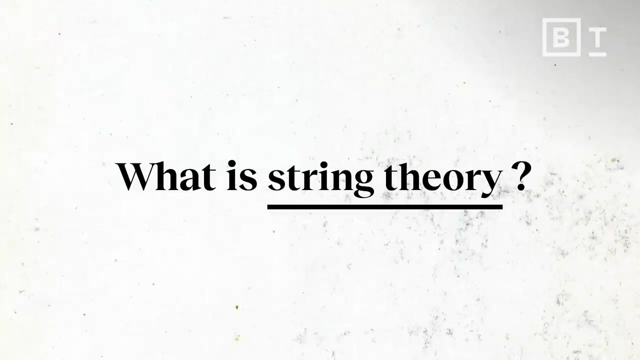 everything. Each one was shown to be anomalous or divergent. So far, there's only one theory which has survived every challenge: String theory, which is what I do for a living. Now, what is string theory? From a distance, an electron? 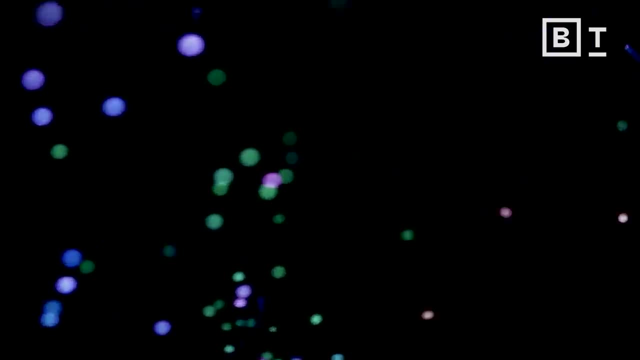 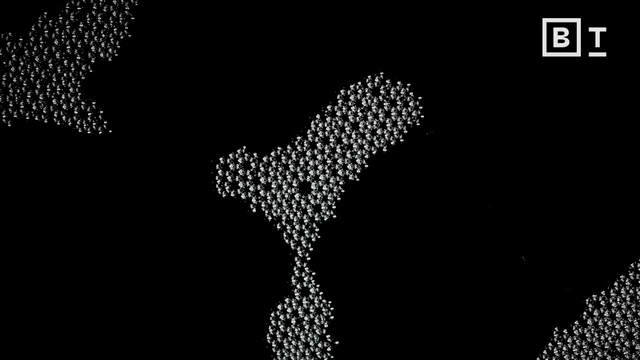 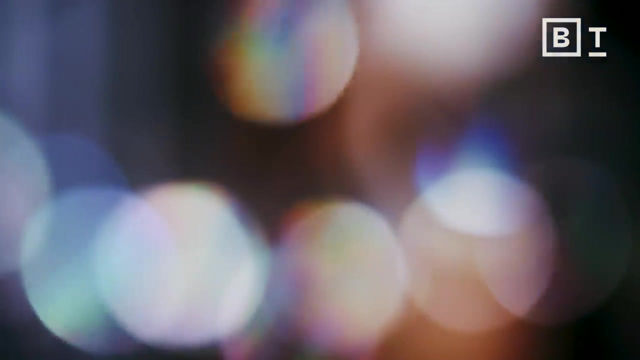 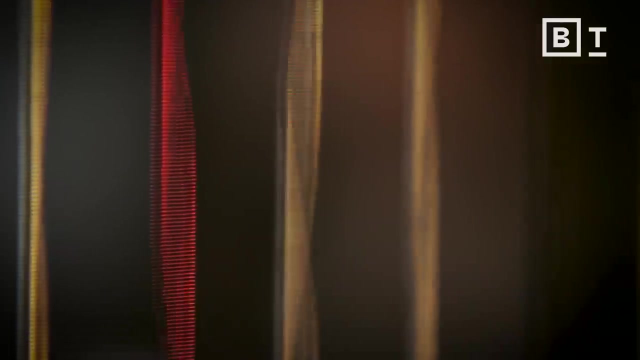 looks like a dot. The neutrino is another dot, The quark is another dot. We have all these dot particles. How many dot particles? Hundreds of them. But string theory says, if you can peer into the heart of an electron, you will see that it's a rubber band, a tiny, tiny vibrating string. 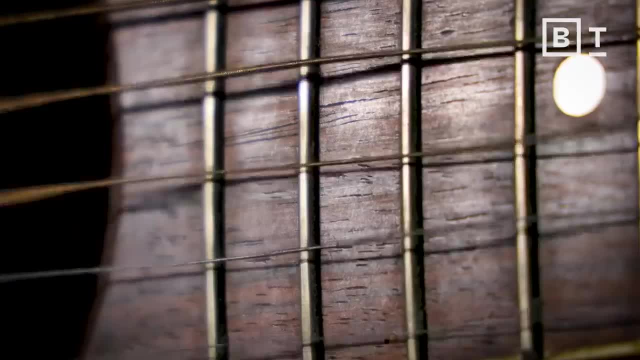 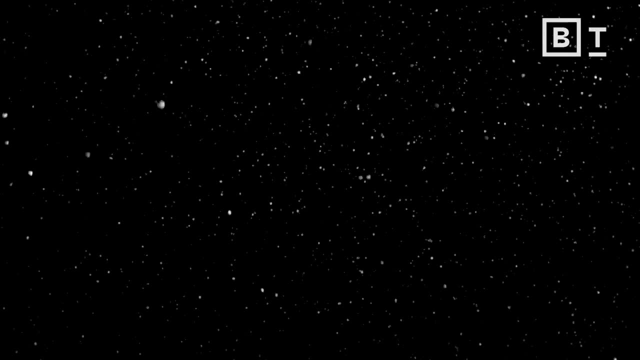 very similar to a guitar string. There's an infinite number of vibrations in a string. There's an infinite number of vibrations in a string. There's an infinite number of vibrations, And that is why we have subatomic particles, The subatomic particles. 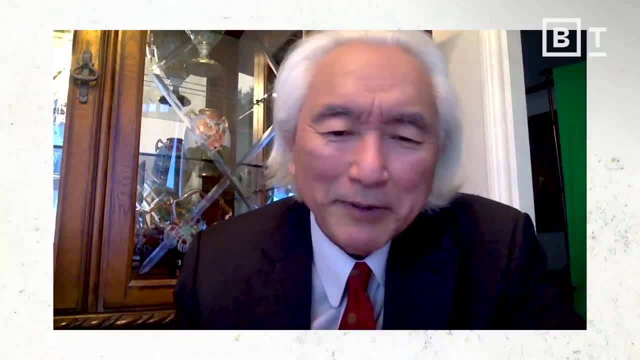 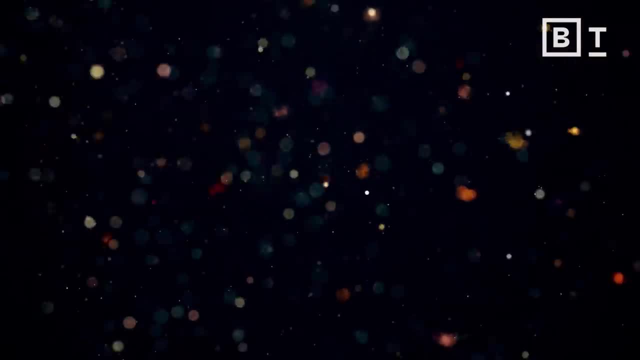 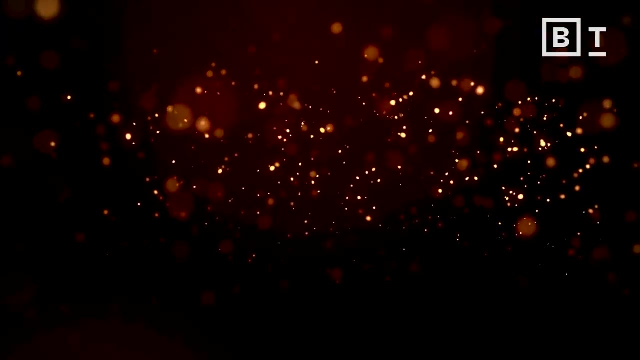 each correspond to a different set of vibrations of a rubber band. String theory allows you to rotate particles into each other, turning electrons into neutrinos, neutrinos into quarks, And the theory remains the same. That is the symmetry of the string, And that's why it's so. 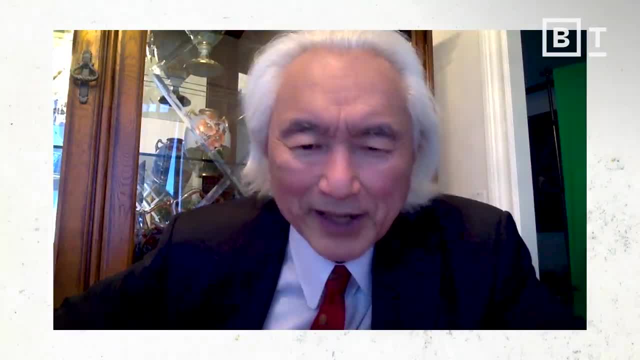 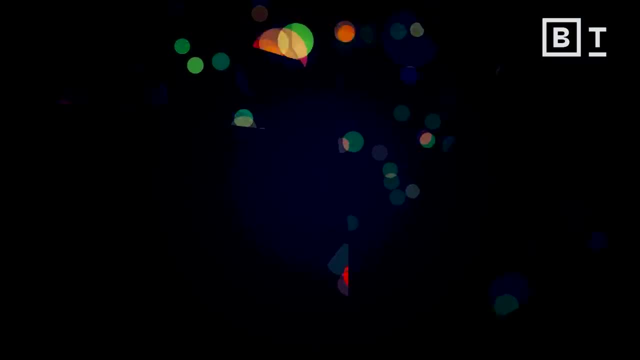 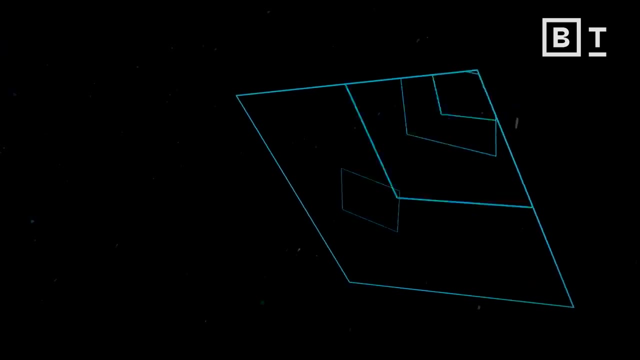 powerful, A simple idea that, in case you don't know, you don't know how to do it, you don't know how to do it. It encapsulates the entire universe. Now, my personal point of view is: string theory is probably the only mathematically consistent theory. All of the theories are mathematically 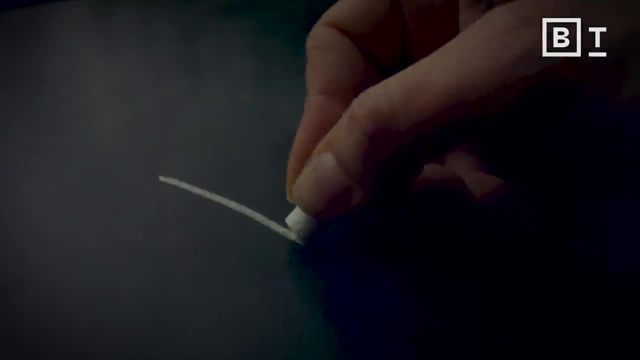 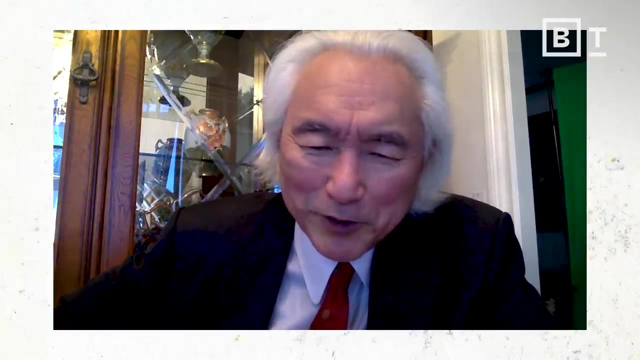 inconsistent. What does that mean? It means that if you prove it far enough, you can prove that 2 plus 2 equals 5.. Therefore the theory is wrong So far. with string theory, 2 plus 2 always is 4.. 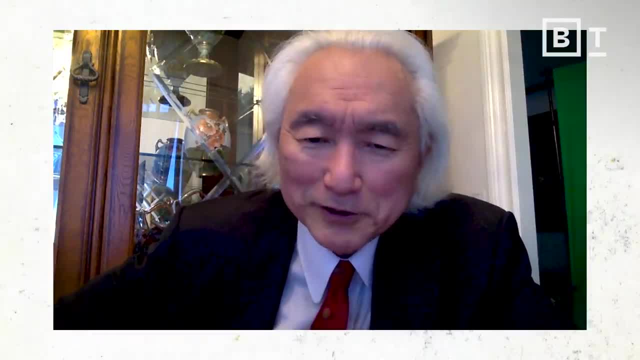 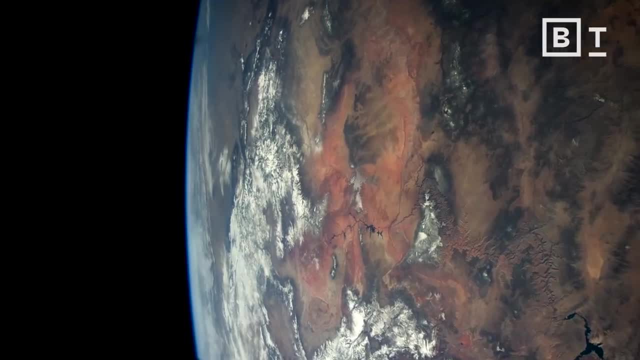 Perhaps it is the only theory Where 2 plus 2 is 4.. There are a lot of objections to string theory. by the way, The biggest objection is: you can't test it. But we're getting closer and closer to being able to.